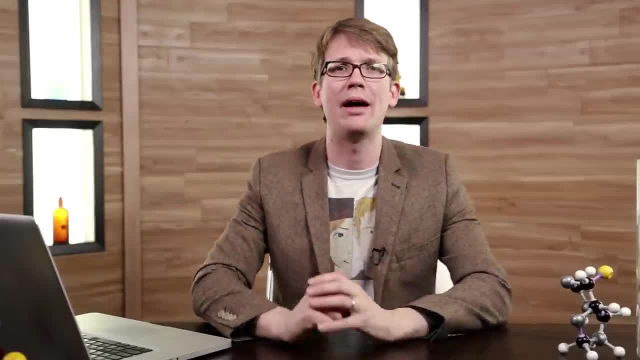 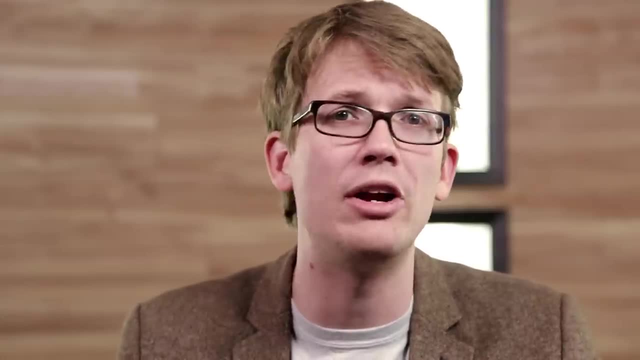 rules that govern some of the world's most useful, or at least used, compounds: the hydrocarbons that we use as diesel fuel- gasoline, methane, propane. You're gonna learn what these and other compounds look like, what their names mean and how they take part in the reactions. 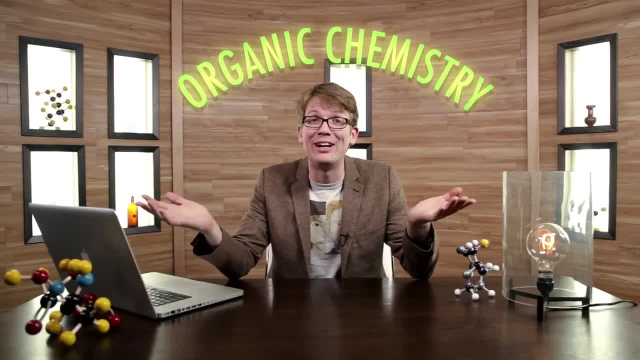 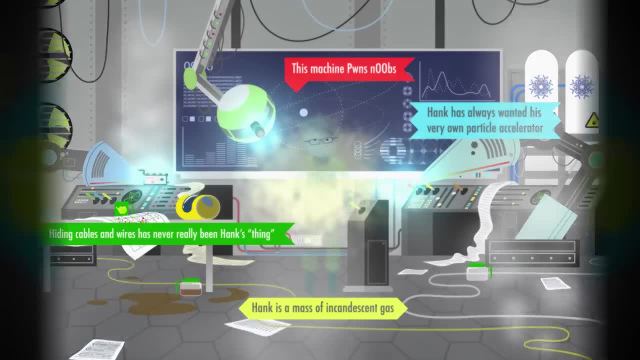 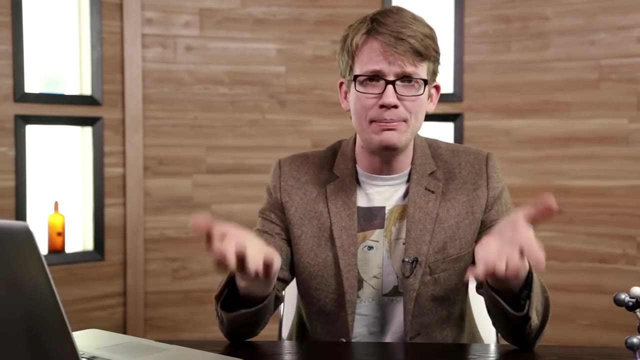 that fuel our lives. Welcome to organic chemistry. INTRO. The fully saturated hydrocarbons I just described are usually called by the much simpler name alkanes. The simplest of the alkanes is one you've heard of before methane or CH4,. 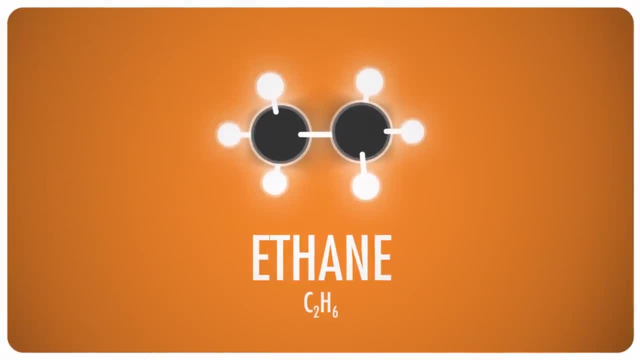 the main compound in natural gas. The next simplest alkane contains two carbons side by side. Each one of them is bonded to three hydrogen atoms. This is ethane, C2H6, another gas, and it's mostly used in the production of plastics. If we add another carbon and 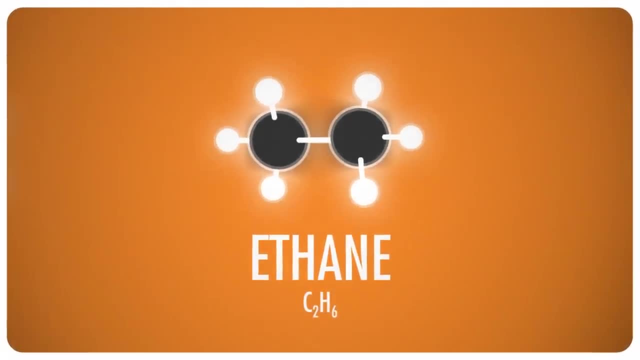 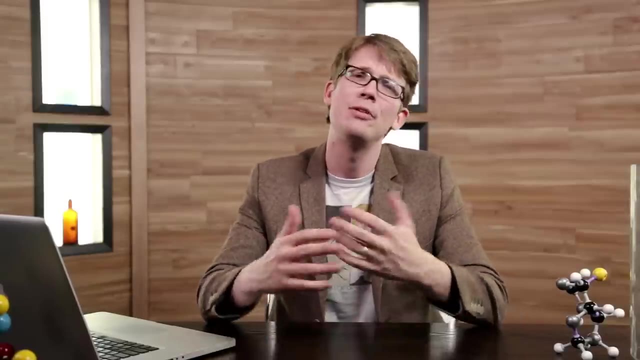 enough hydrogens to fill all those spaces. we get our next alkane propane C3H8.. Also a gas at room temperature and normal atmospheric pressure, propane is a common fuel for cooking, heating and vehicles, as well as a propellant for everything from aerosol cans to paintball. 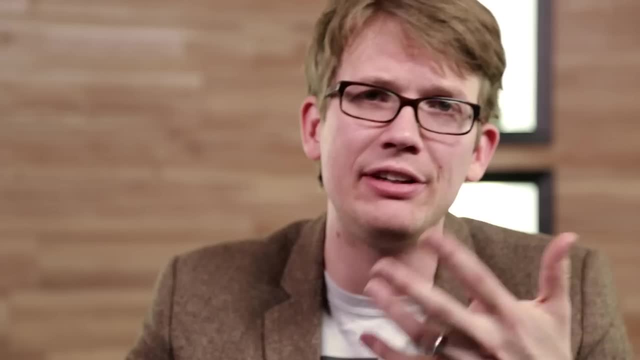 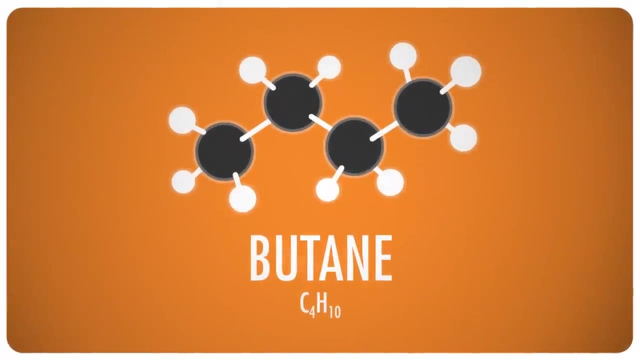 guns, And we could do this all day, adding carbons to the chain and giving each compound a name, but that would be pretty boring. Things get more interesting, though, with the next alkane INTRO. Butane C4H10,, because there are two different forms of it. The first is what you'd expect. 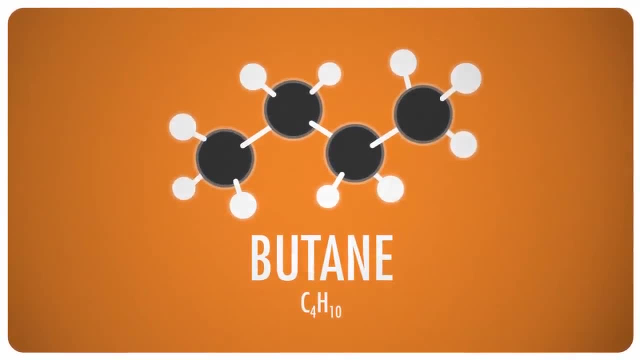 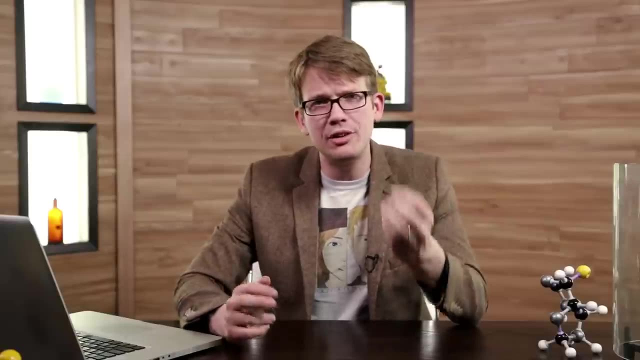 just a chain of carbons with hydrogen stuck wherever they're needed to make. each carbon have four bonds. This is called normal butane or n-butane. But you can also arrange the four carbons differently by making a chain of three and then branching the fourth one. 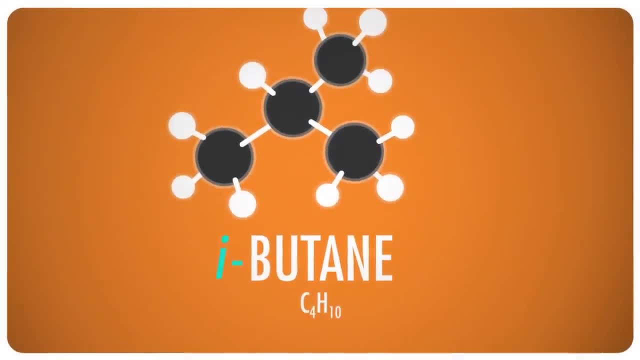 off the center of the chain. This is called isobutane or i-butane, and even though it has the same chemical formula as n-butane, its structure gives it different properties. For example, n-butane is the same chemical formula as n-butane. 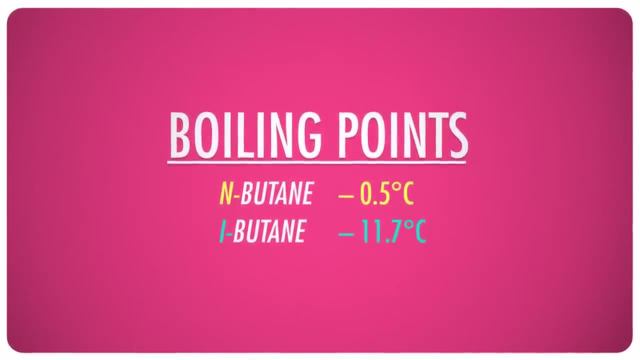 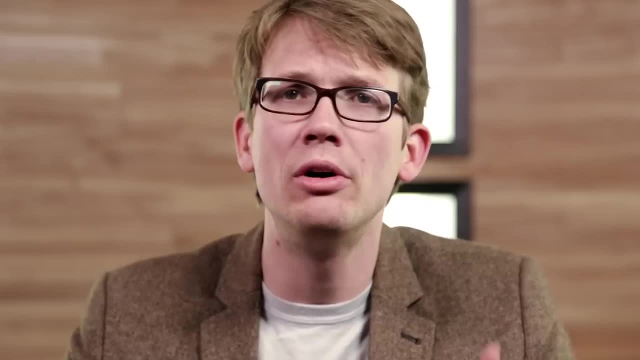 N-butane boils at negative 0.5 degrees Celsius, while isobutane boils at negative 11.7 degrees Celsius. These different structures for compounds that have the same molecular formula are called isomers. As you add more and more carbon atoms to the molecule, there are more and more ways. 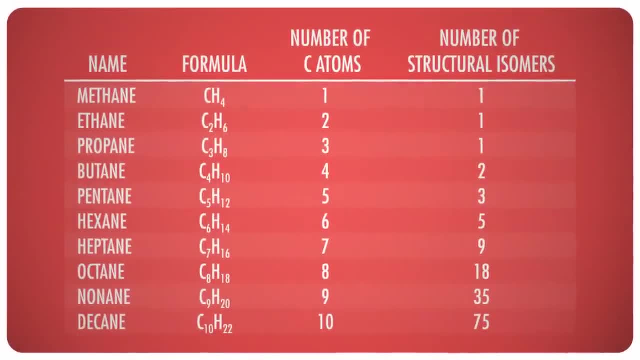 that you can arrange them. So the number of atoms in butane only allows for two isomers: n-butane and isobutane. But pentane, or C5H12, has three possible isomers, and C6H14,, known as hexane, has five. 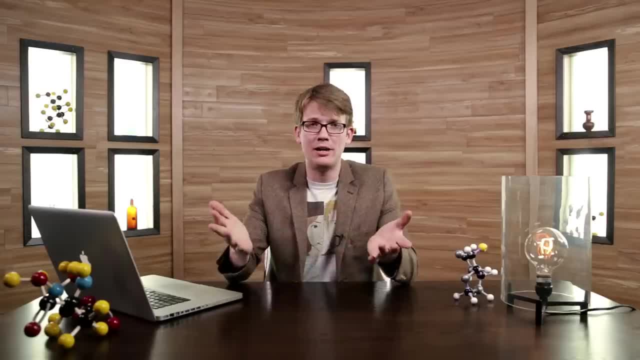 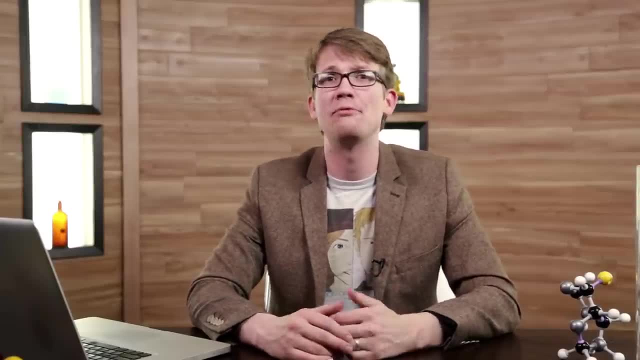 Again, I could do this all day, But looking at this table of the number of possible isomers, you can see that that escalated quickly. The takeaway here is that molecules with the same mass and number of atoms can form different structures, and as their structure changes, their properties also change. 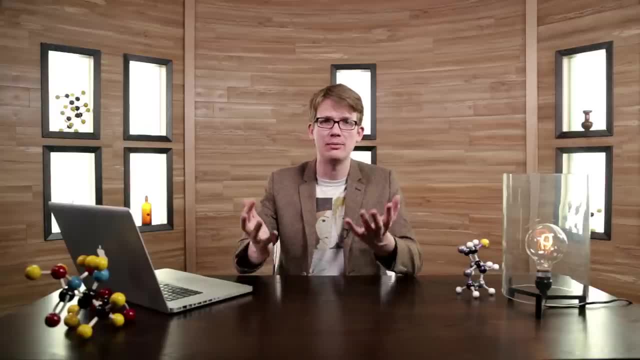 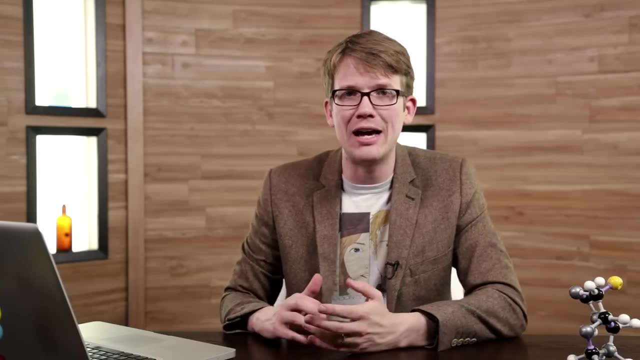 As a general rule, the larger and more complex alkanes are, the more densely their molecules can pack together, which means that they tend to be liquid or solid instead of gaseous at room temperature. So alkanes with main chains of five to eighteen carbon atoms, like octane and gasoline, are 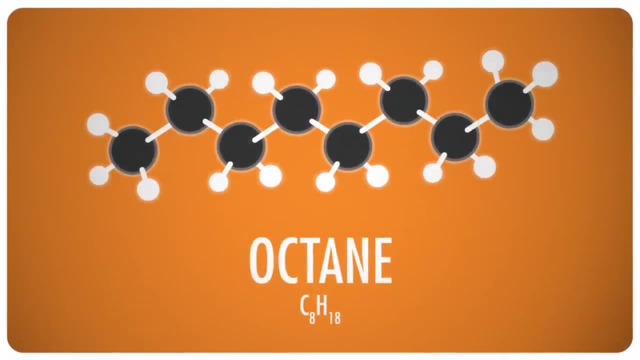 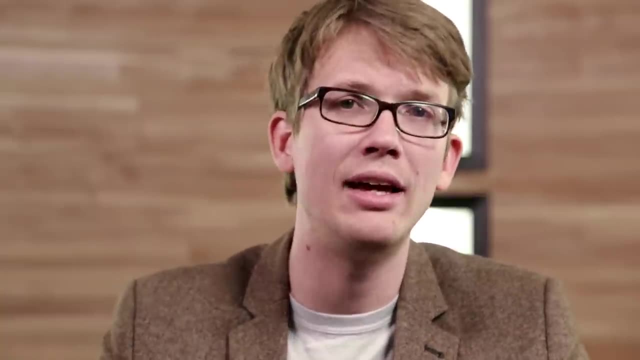 liquids at room temperature and those with more than eighteen carbon atoms, like paraffin or other waxes, are solids. Now you're probably picking up on a lot of words that you've heard before, even outside of chemistry class Octane, propane, methane, paraffin, so on. You can chalk that up to: 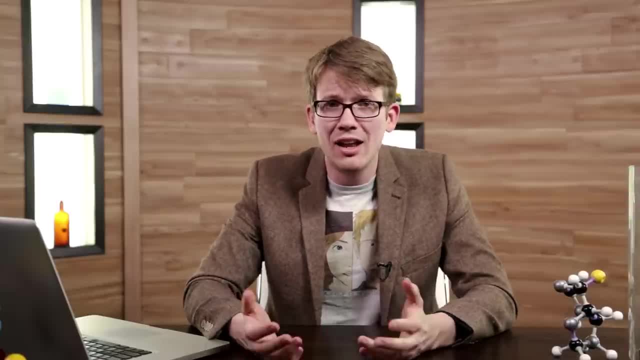 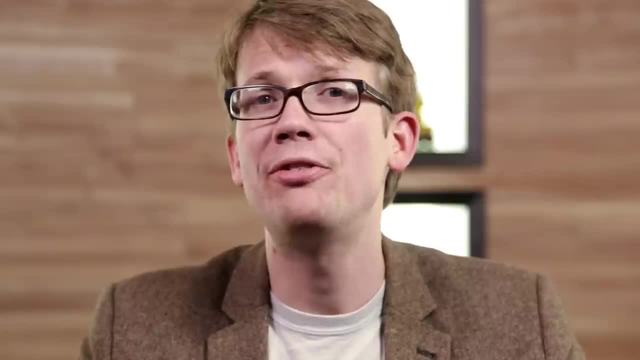 the enormous popularity of these compounds in our daily lives. Like I said, hydrocarbons are super useful because of the types of reactions they can take part, in which I will explain more in a bit. But first I think it's high time you know what these names actually mean, Much like. 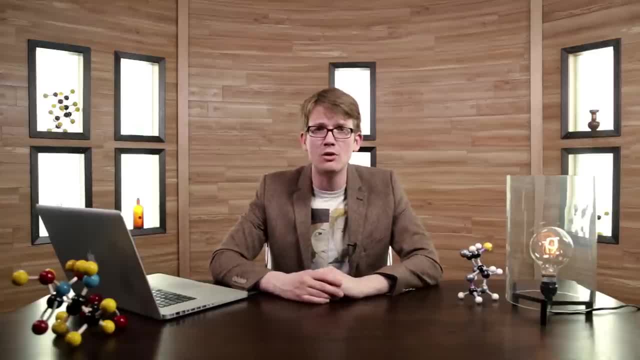 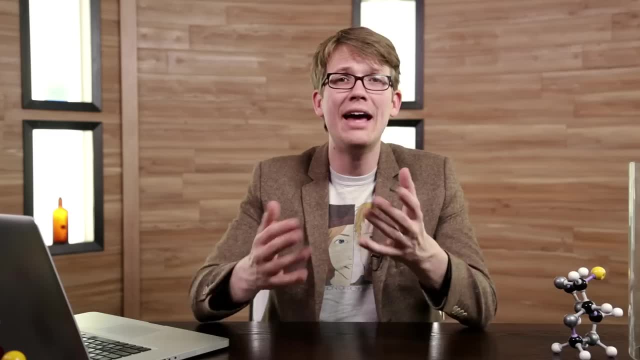 the general language of chemistry that we talked about months ago. organic nomenclature has its own system of prefixes, suffixes and numbers that tell you what's in the compound being named. Now you gotta know the prefixes, because they indicate how many carbon atoms are present. 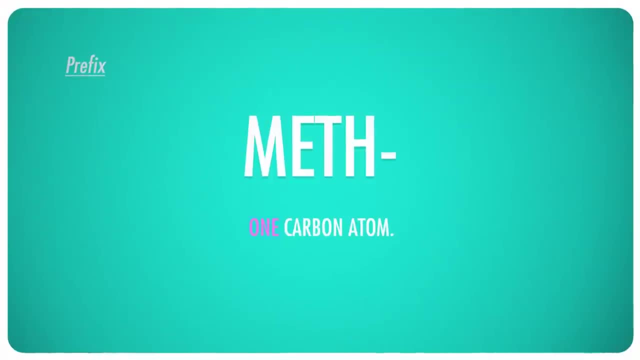 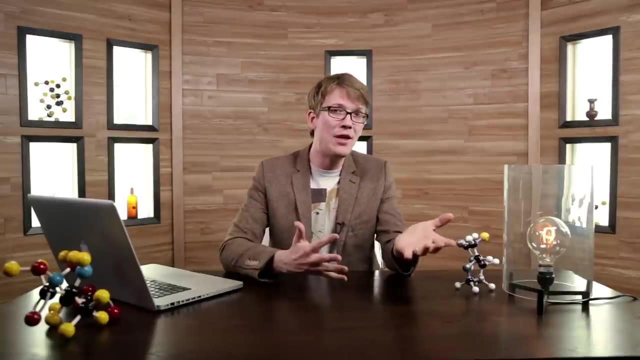 Here's one that I know you've heard before: Meth. Meth in a name always indicates a molecule or branch containing one carbon atom. So the difference between amphetamines that doctors prescribe and methamphetamines that are sold on the streets is that methamphetamine 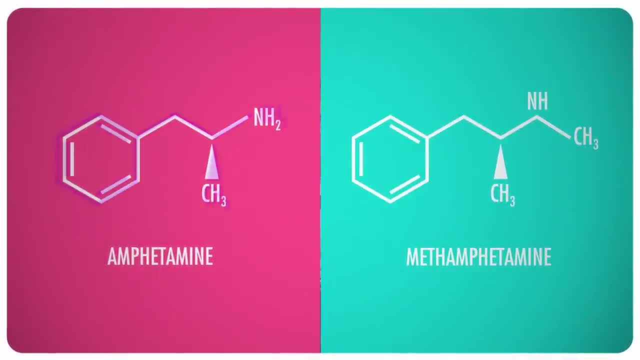 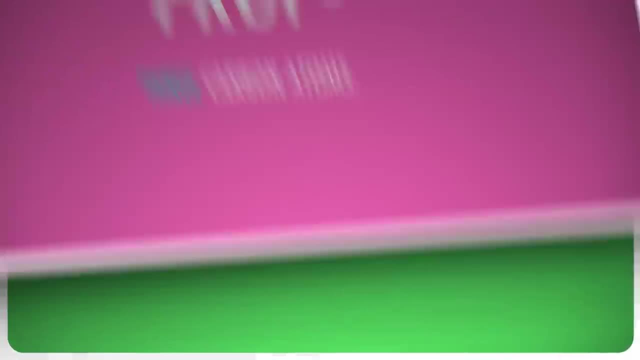 has a methyl group, CH3, with one carbon, where amphetamine just has a single hydrogen atom. That's helpful to you. Don't do drugs. Eth, meanwhile, indicates two carbon atoms. Prope means three, Bute means four. 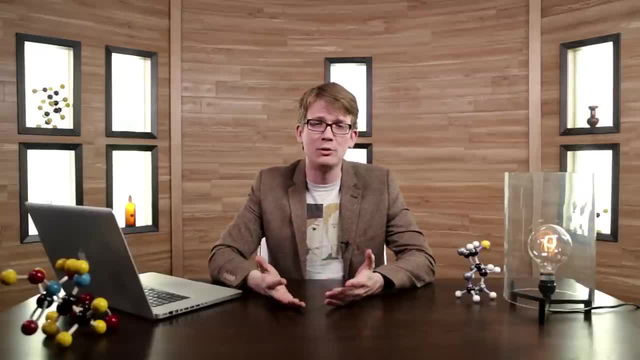 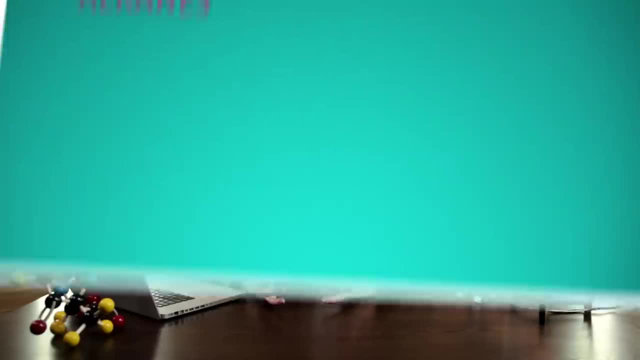 From there, most of the prefixes will be familiar from geometry class and you can review them in tables and learn them. I'm not going to go through it all Now. there are a few naming rules that are specific to alkanes. First, alkanes are always. 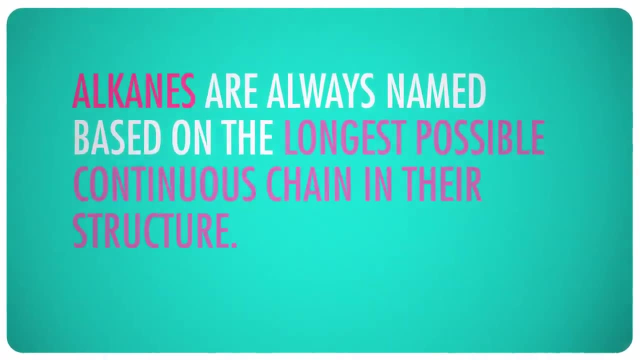 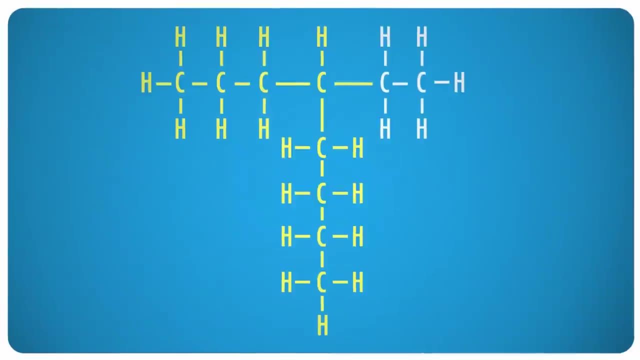 named based on the longest possible continuous chain in their structure. For example, even though this looks like a five-carbon chain intersecting with a six-carbon chain, it actually contains an eight-carbon chain, So this is considered an octane with a two-carbon chain attached to one of its carbon atoms. 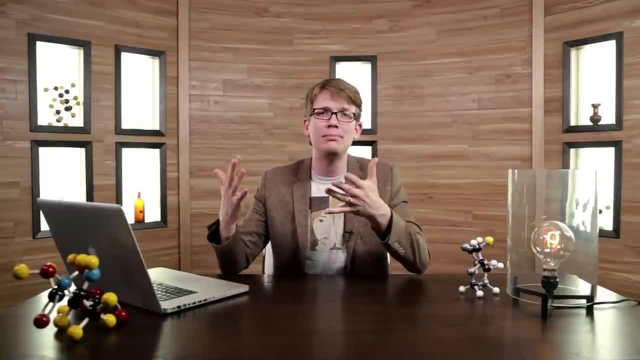 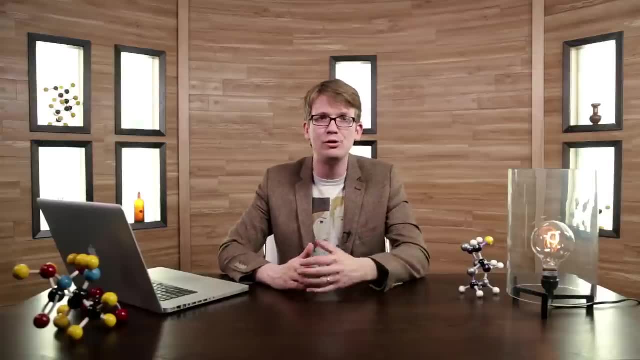 When shorter carbon chains are attached to longer ones like this, they're still named using the same prefixes, but we stuff a little y-l onto the end to show that they're just attachments. Since this attachment has two carbons, we call it an ethyl group And the 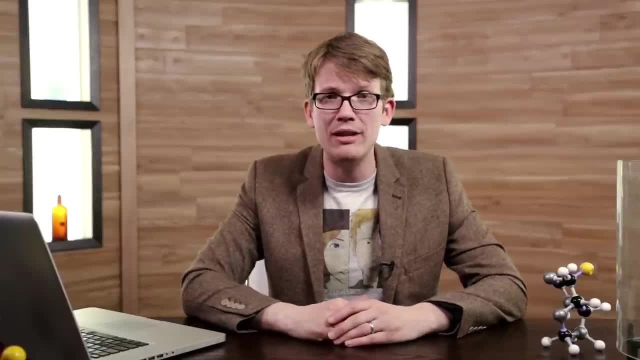 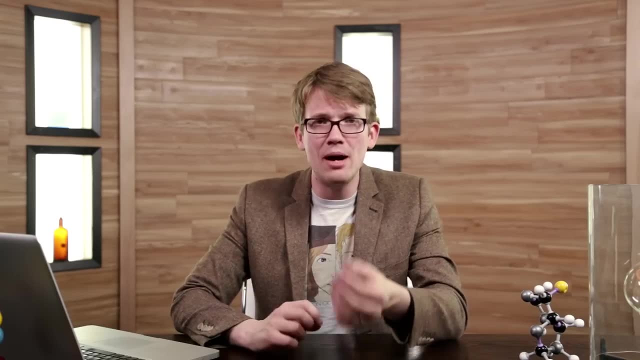 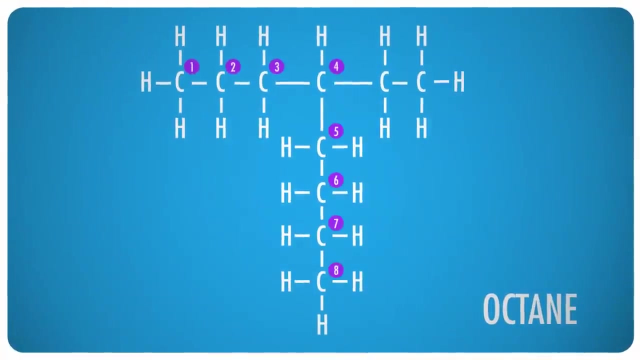 attachment with just one carbon that turns amphetamine into methamphetamine. that's a methyl group. Attachments are also given a number to show you where along the chain they're attached. The long chain is always numbered carbon-by-chain, So if we number the chain the right way, the ethyl group will end up at position four. 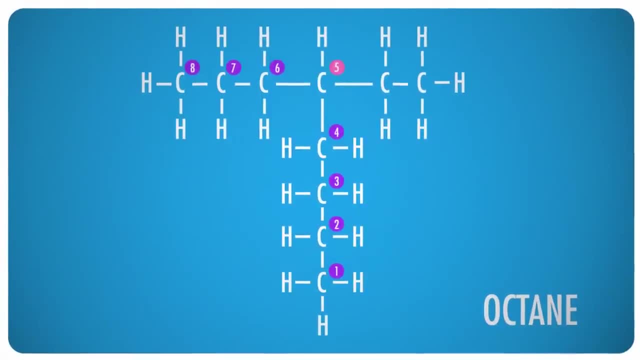 But if you do it the wrong way, it's in position five. Low numbers win, So it's numbered from left to right in this case. So when we put it all together, this compound is called 4-ethyl-octane. Congratulations. 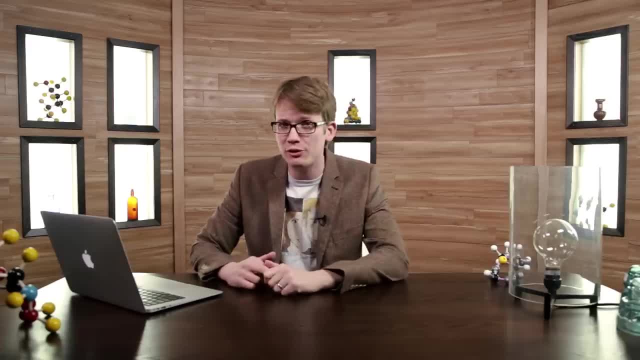 you just named an organic compound. Now, particularly astute and studious students will have noticed something here. Earlier, I introduced you to isobutane, a compound with four carbons that were non-organic, And this compound is called 4-ethyl-octane. So, if we put it all together, this compound is called 4-ethyl-octane. Congratulations, you just named an organic compound. So if we put it all together, this compound is called 4-ethyl-octane. And this compound. 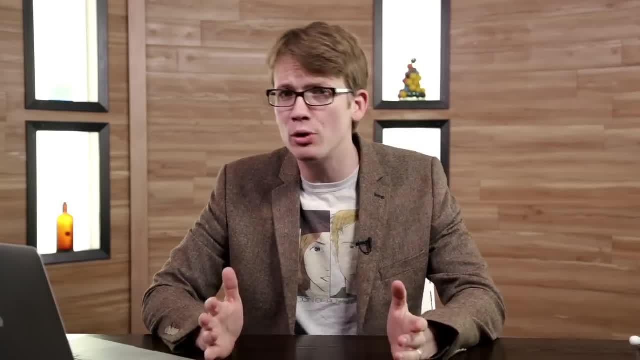 is actually called 4-ethyl-octane, But it's not all in a chain. We call that isobutane and it is an isomer of butane, But according to these all-important rules of nomenclature, it's not actually any sort of butane at all. 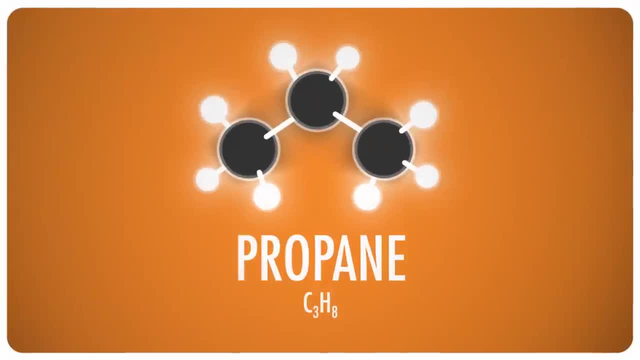 The longest carbon chain is just three carbons long, So it's propane with one methyl group sticking off of it. If we wanted to give a technical name to it, isobutane would be 2-methyl-propane Though. 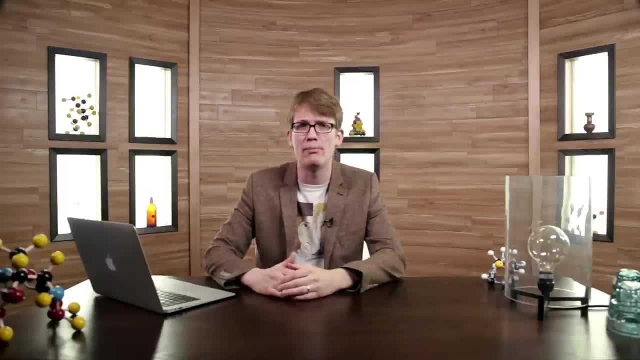 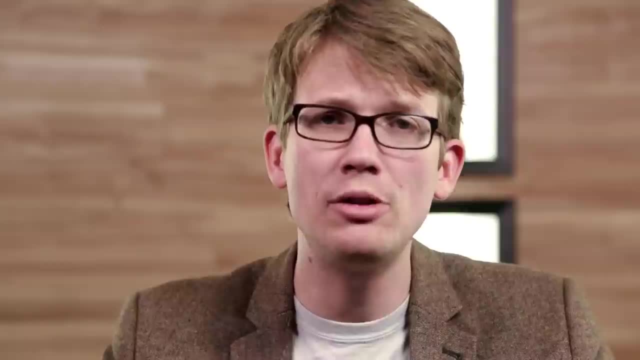 since the second carbon is the only place where the methyl group can go without the molecule once again becoming butane properly, proper chemists just drop the 2, and call it methyl-propane. Now suppose you have more than one of the same size group attached to the same chain? 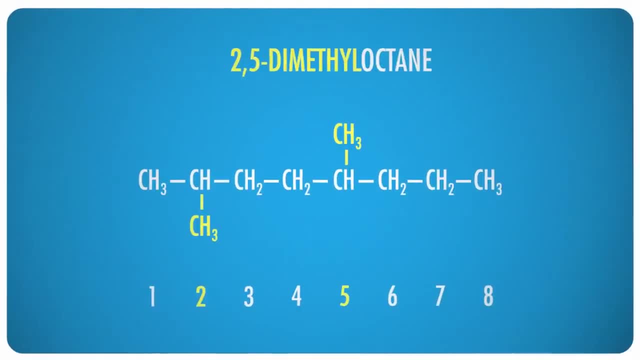 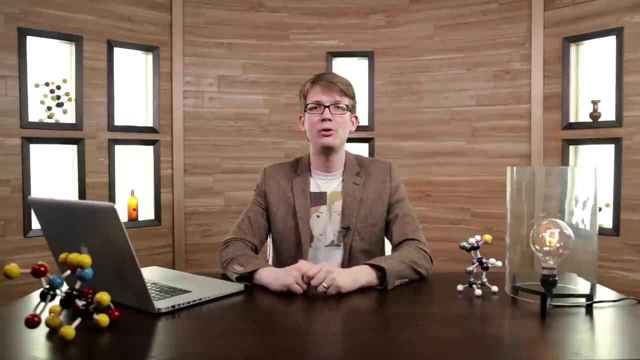 like two methyl groups on the same alkane. In this case you put a number for both of them, and then prefixes like di and tri are used to indicate the multiple attachments. So, for instance, if an octane chain has methyl groups attached to its second and fifth carbons. 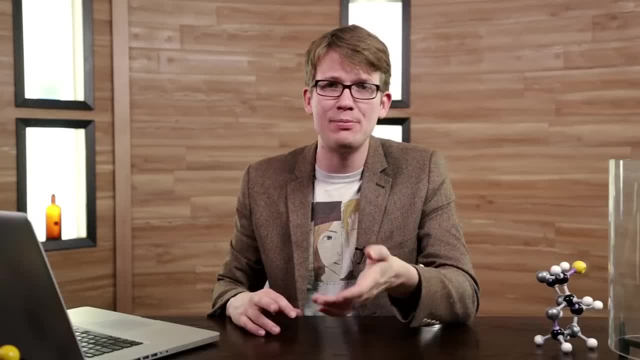 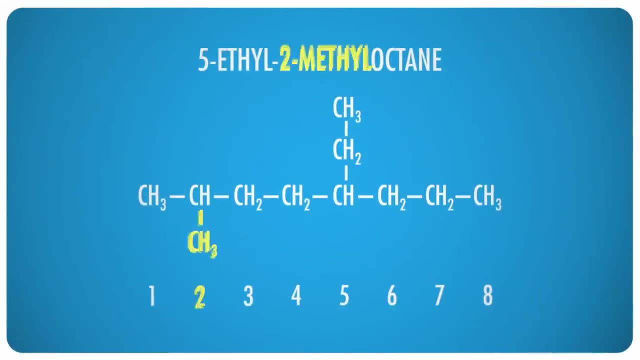 it's called 2,5-dimethyloctane. On the other hand, if you have attachments of different lengths, you just name and number each one separately, being sure to list them in alphabetical order. So if the structure we just used had a methyl group on its second carbon and an ethyl group, 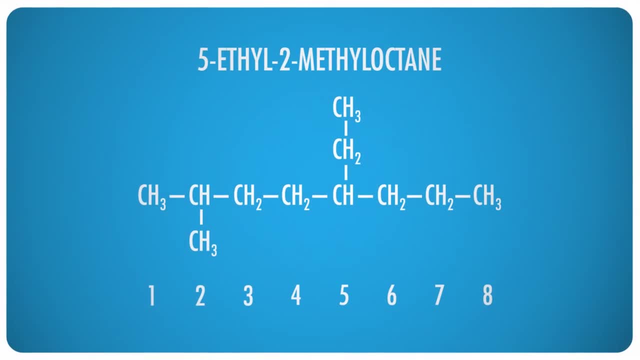 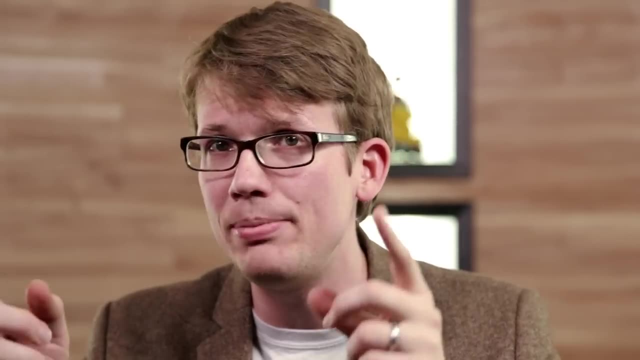 on its fifth, it would be 5-ethyl-2-methyl-octane. This is super useful for several reasons. One, because there are trillions of ways that organic compounds can come together, but also because you can work backward from a name and build a structural formula from it. 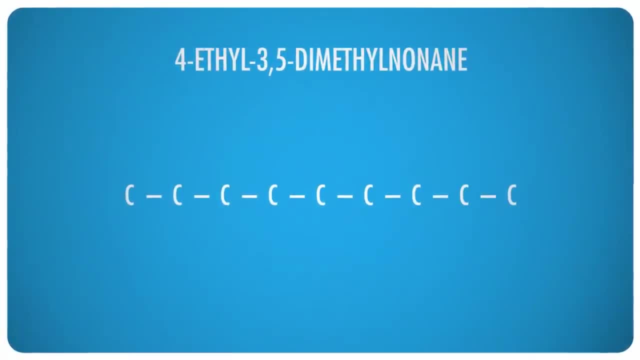 Let's try that out. We're going to build 4-ethyl-3,5-dimethyl-nonane. Start with the main chain nonane. The prefix non- indicates nine carbons. Then add an ethyl group, a two-carbon chain on carbon, number four. 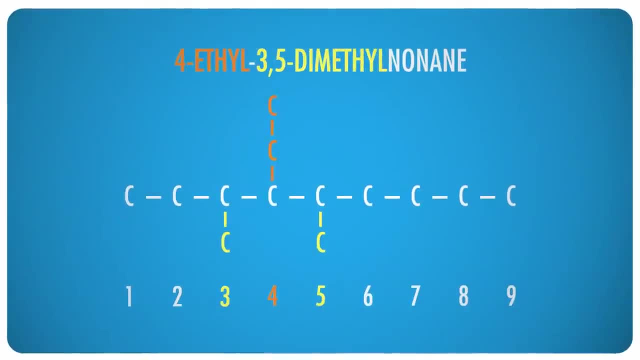 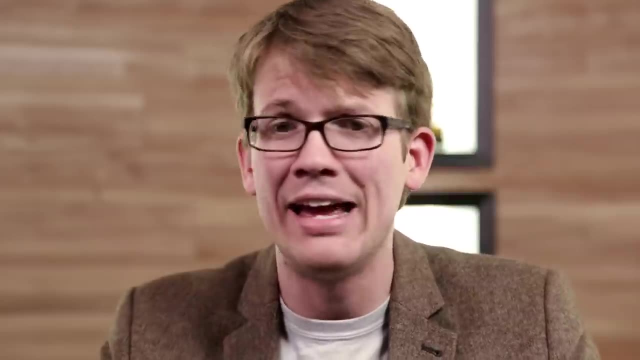 And then methyl groups: just one carbon on carbons three and five. Our final step is to add enough hydrogen atoms to give every carbon atom four bonds, And now the molecule is complete. It's like a puzzle that we got to make. 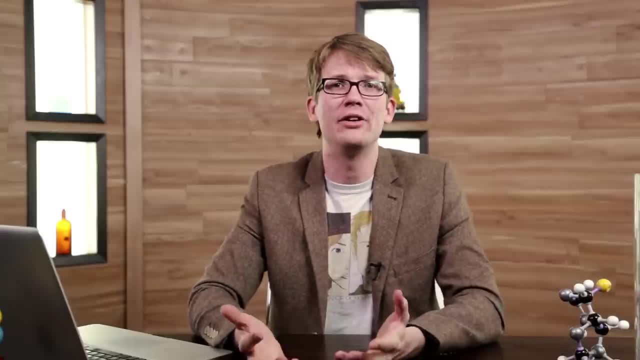 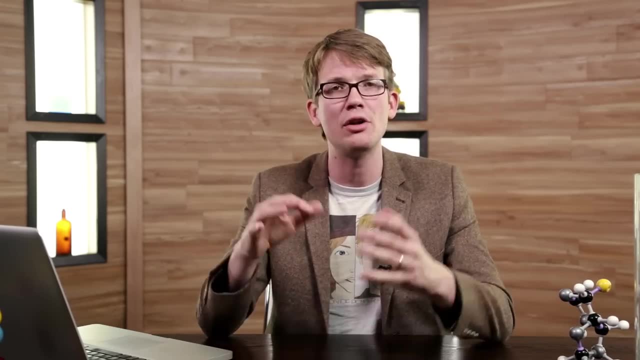 Of course, these compounds don't exist in isolation. Like any other compound, they can undergo a whole variety of reactions, But there are three types of alkane reactions that are important enough for us to cover right now, right here. The first is the kind that hits you first. 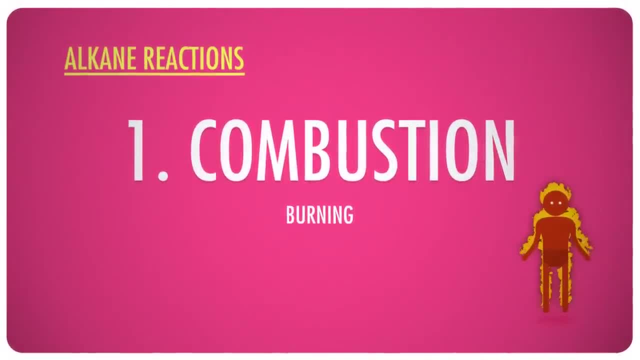 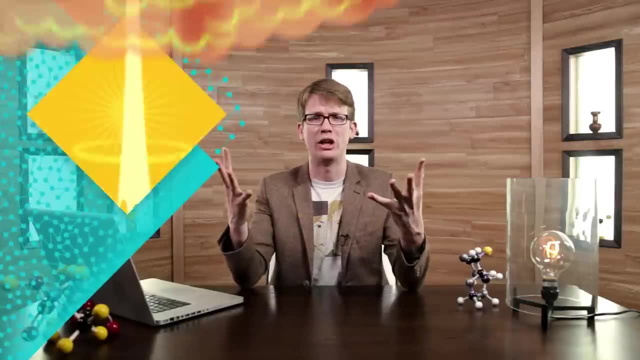 The kind that has made alkanes the most common fuels for combustion or burning. You'll note here that I'm saying burning. A common misperception, even among chemistry students, is that combustion somehow equals explosion. While that would definitely make things more interesting, also more dangerous. those two 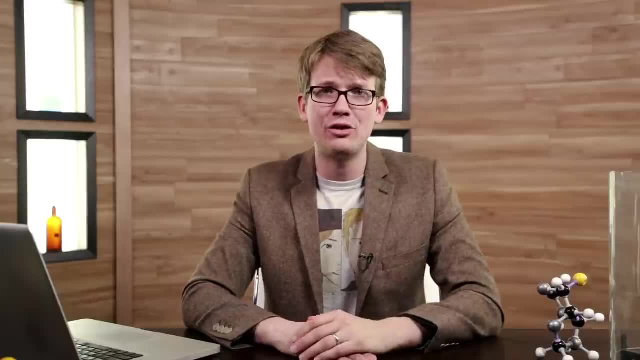 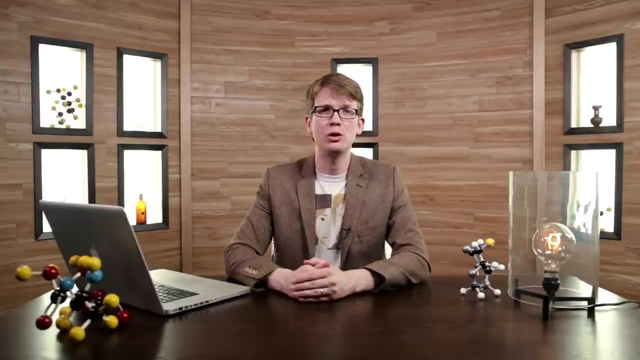 things are not synonymous. Combustion is the type of reaction that powers your car and your propane grill, even candles, among many other alkane fuels. The general reaction for combustion requires a hydrocarbon oxygen gas and a source of heat energy. 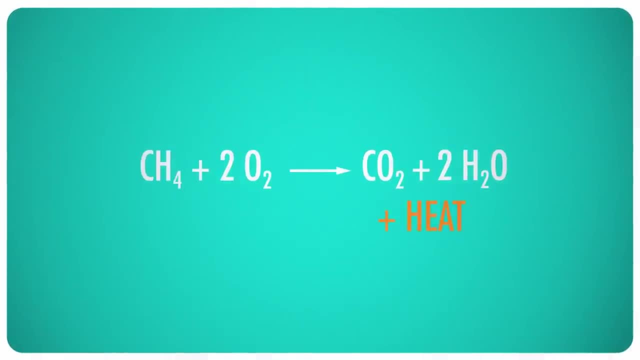 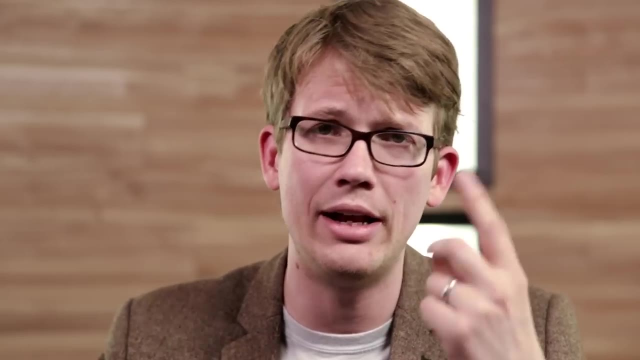 For example, we're using methane, but it works the same for any pure hydrocarbon. The only thing that changes is the coefficients. The products of the complete combustion of a pure hydrocarbon are always carbon dioxide and water vapor. Just those two things. 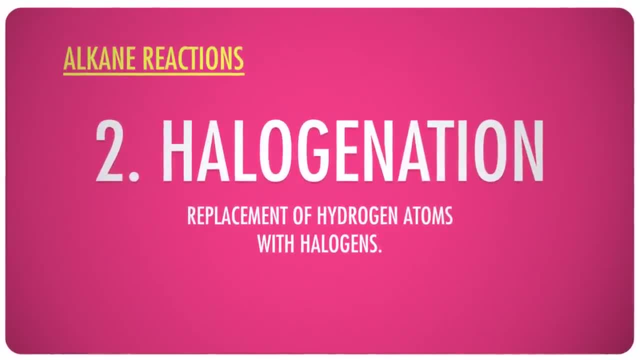 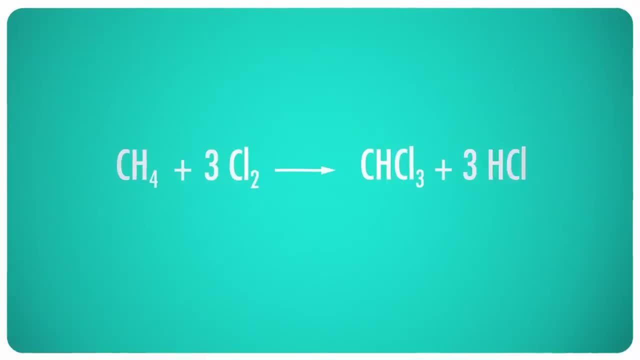 The next major type of reaction that alkanes experience is halogenation, when halogen atoms like fluorine or chlorine are substituted for one or more hydrogen atoms. in the alkane, For example, the rather well-known compound chloroform is more correctly called trichloromethane. 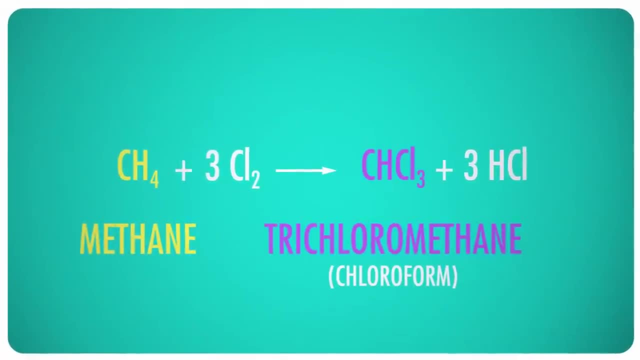